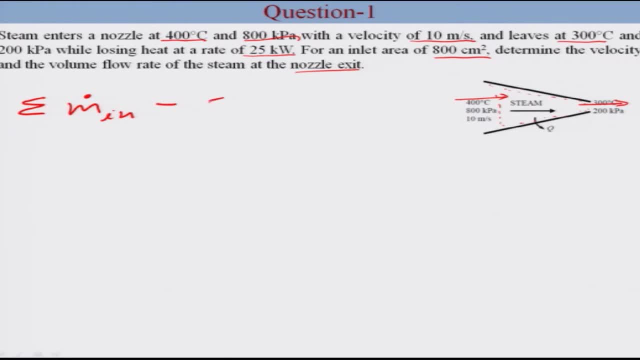 of mass in minus total rate of mass out of the system will be equal to total change in mass of the system, Since this is a steady state process so nothing will change with time. So delta m will be 0 of the system. That means mass flow rate coming in will be equal to mass. 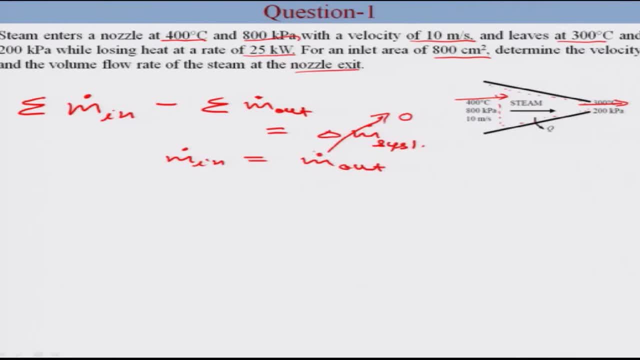 flow rate coming out of the system and let us say it is equal to m dot. Now, from the energy balance on this system we get rate of energy in and out of the system. So this is how I get the rate of energy in. so this is the maximum volume and oxygen when done. 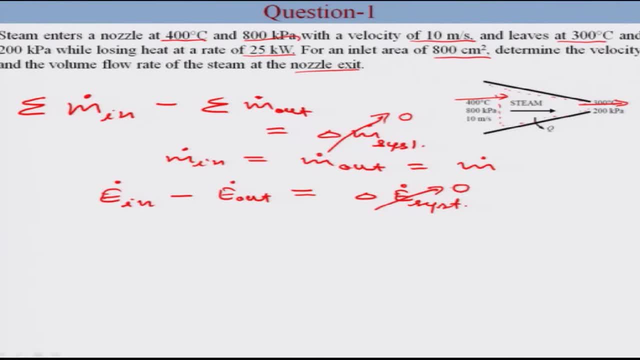 one by one, this is equal to m o R by T. This would be m dot. The current amount of energy that is coming in from the detected Luna will be equal to m o R by 30 powers. � weekend in is equal to 10 for fact f other. So, 1 to the power in minus rate of energy out will be equal to change in energy of the system. So since this is steady state process, it will be 0: н and from here we get rate of energy in will be equal to rate of energy out. N. Monomeris N, Section 1, N12ía In Ð, from here we get time, here 1, where total energy när. 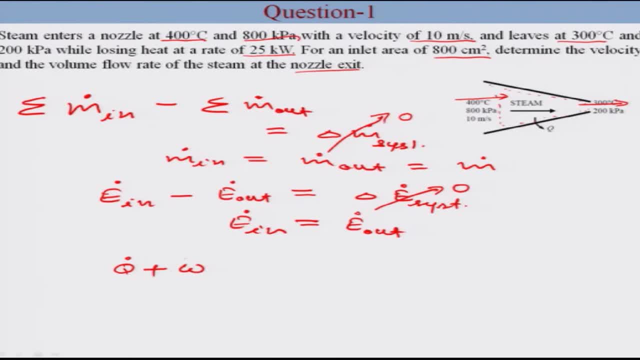 heat coming in plus shaft work, total energy of the flowing fluid in will be equal to heat coming out of the system, plus work coming out of the system, plus again total flow energy of the fluid coming out of the system. since nothing is going in, no energy is since no energy is going. 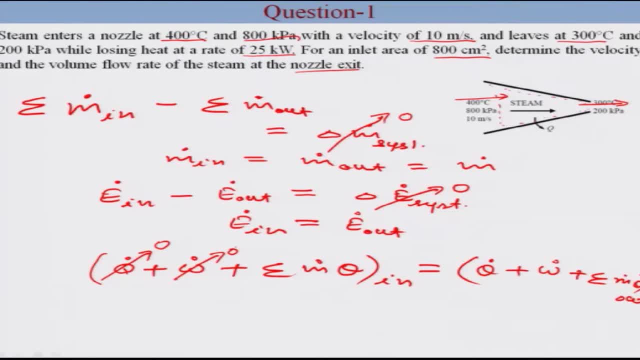 in the system. no shaft work is there in the system, so these two terms will be 0 and same. there is no work done by the system, so this w dot will also be 0.. so from here we get mass flow rate, times, flow, energy of fluid coming in the system will. 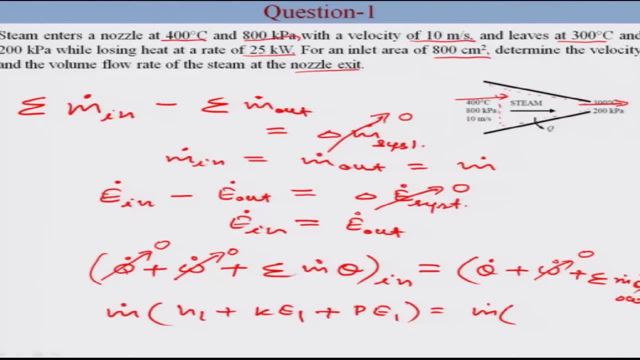 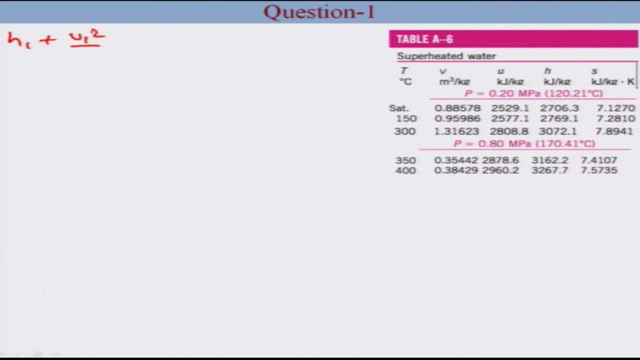 be equal to mass flow rate times flow energy of fluid coming out of the system plus heat coming out of the system. so after solving this we get h 1 plus v 1 square by 2 equal to h 2 plus v 2 square by 2 plus q, out upon m dot, assuming here that delta p equal to 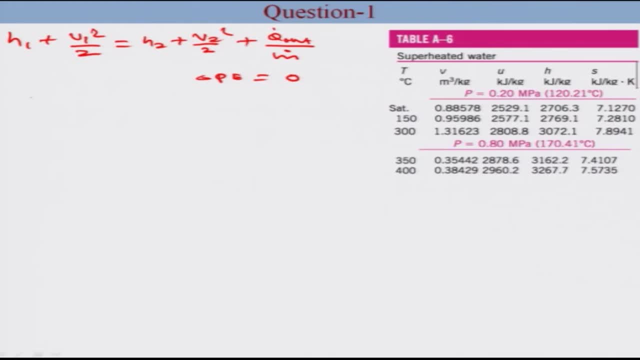 0.. so from here we need to find exit velocity. that is v 2. so after solving this we get h 1 minus h 2 plus v 1, square by 2 minus q dot out upon m dot. so this is our first expression. 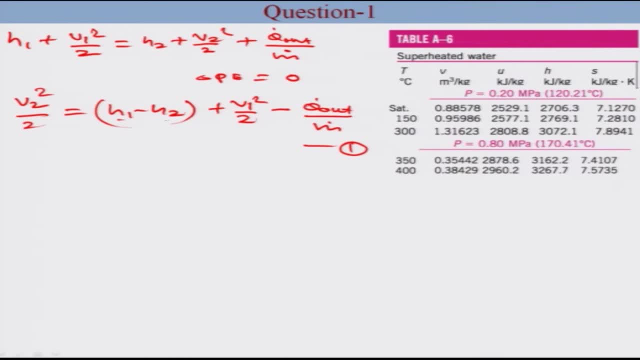 so in order to get v 2, we need to know h 1, h 2 and mass flow rate, since v 1 we know and q out we also know. ok, so it is given that at inlet condition, p 1 equal to 800 kilo pascal and t 1 equal, 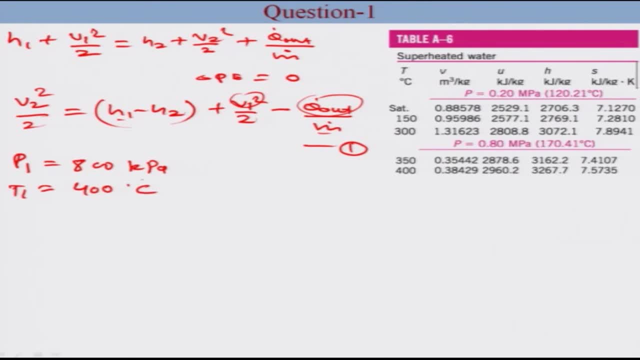 to 400 degree centigrade. at this condition, saturation temperature should be 170.41 degree centigrade, but here this t 1 is greater than t saturated. that means this condition is superheated. ok, so we need to look into superheated water. 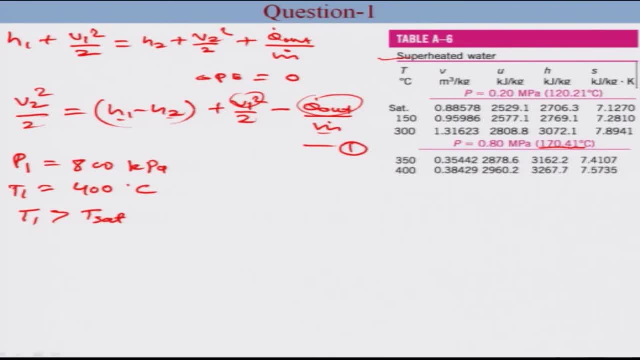 table to get this h 1 and h 2.. so from here we get specific volume at 400 degree centigrade and 800 kilo pascal, which is nothing but 0.8 mega pascal. so v 1 will be 0.38429.. 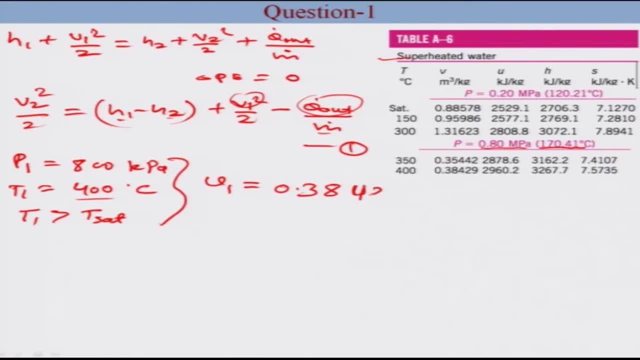 ok, which is this value? meter cube per kg. similarly, inlet enthalpy, 3267.7 kilo joule per kg at this 400 degree centigrade and 800 kilo pascal. which is this value. so at the exit it is also given that p 2 is 200 kilo pascal and t 2 is 300 degree centigrade. 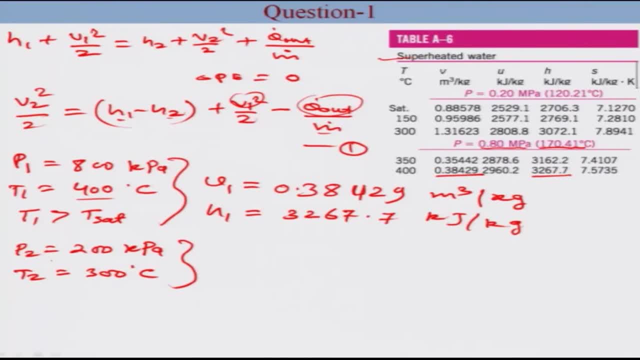 so corresponding to this conditions. this condition is also at superheated condition because t 2 is greater than t sat, because t sat should be 120.21 degree centigrade. ok, at this 200 kilo pascal, but this temperature is above this t saturation temperature. 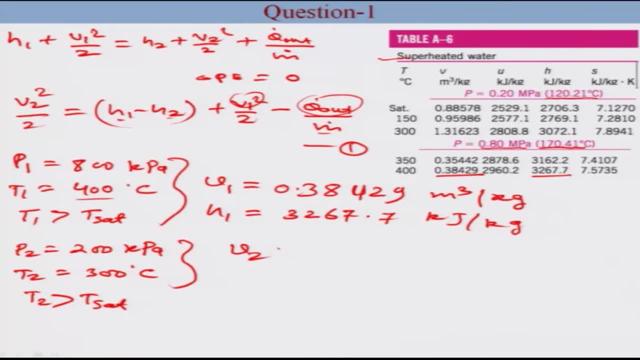 so corresponding specific volume v 2 will be equal to 1.31623 meter cube per kg, which is this value, and corresponding enthalpy h 2 will be 3072.1 kilo joule per kg. ok, so this value. now we need to find mass flow rate, ok. 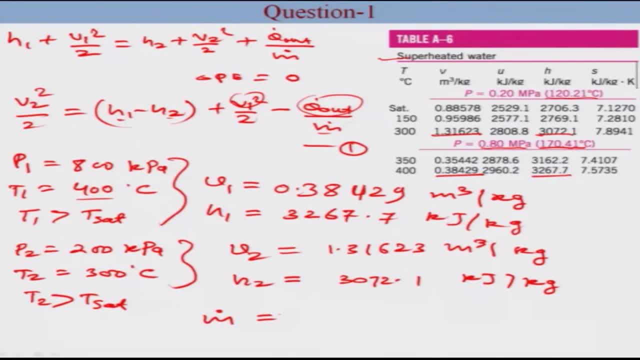 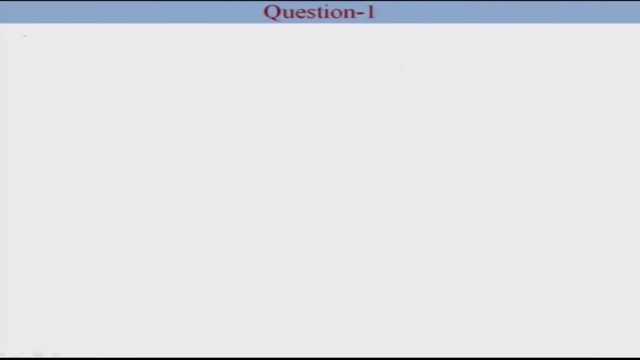 so the mass flow rate can be calculated as inlet area, inlet velocity divided by initial specific volume. ok, so after plugging these values here, we get m dot equal to m dot, equal to m dot equal to 0.08 meter square. it is given in the problem. velocity is also given 10 meter per second. 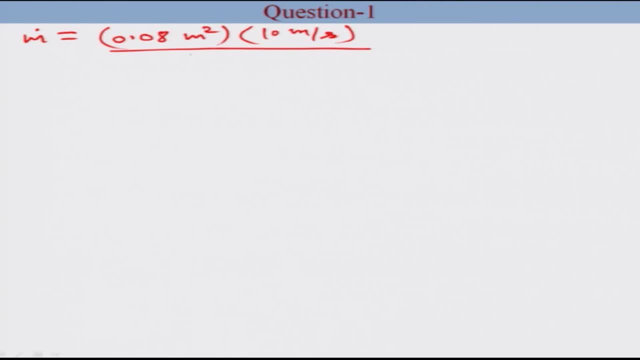 and specific volume that we have calculated right now: 0.38429 meter cube per kg. so this gives us 2.082 kg per second. ok, so this gives us 2.082 kg per second. ok, ok, ok. 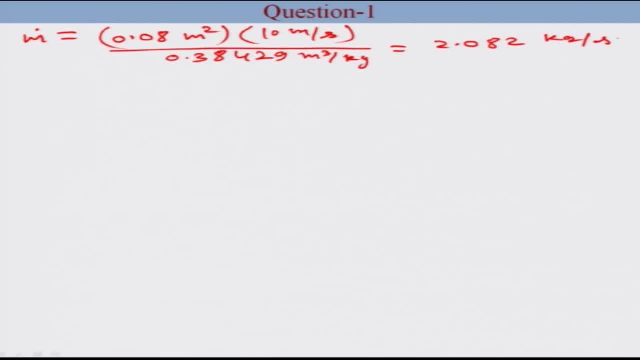 ok, ok, substitute these values in equation 1, we get v 2 second by 2, equal to h 1 minus h 2, which is 3267.7. minus h 2 is 3072.1 kilo joule per k g plus v 1.5. Benjamin Music is here. 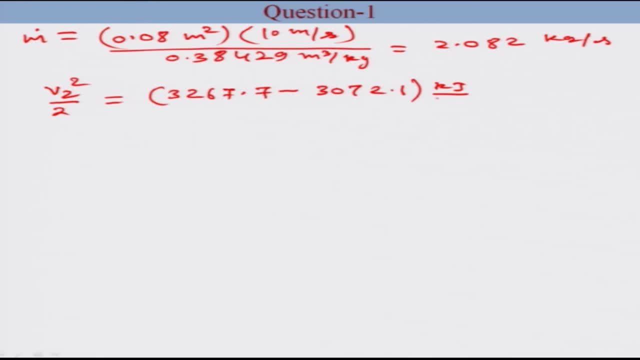 v 1 e two square by 2, we have gave equal 1.7.. freeóstom in equation: 2 per kg plus V, 1 square by 2, which is 10 meter per second by 2.. We have to convert it into: 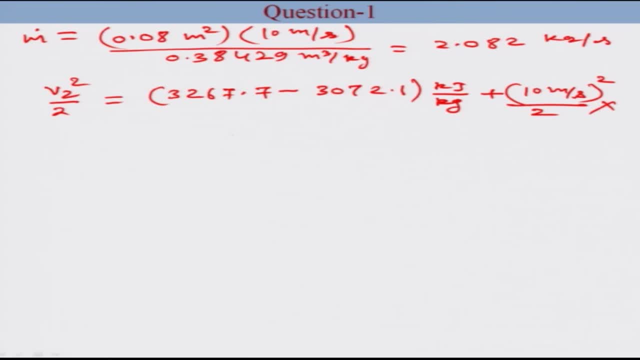 energy unit. So multiplied by since 10 to power, 3 meter square per second square is equal to 1 kilo joule per kg minus Q out upon m. So Q out is given in the problem, which is 25 kilo joule per second, and m dot that we have calculated here 2.082 kg per second. 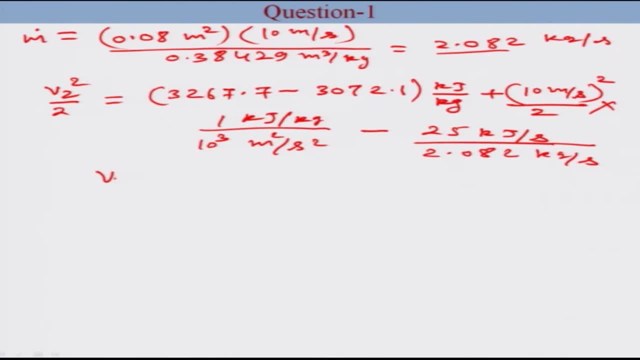 So after solving it We get V 2 equal to 606 meter per second. So further we need to calculate volumetric flow rate at the exit, So that will be equal to mass flow rate times specific volume at exit. So after putting these values here, 2.082 kg per second. 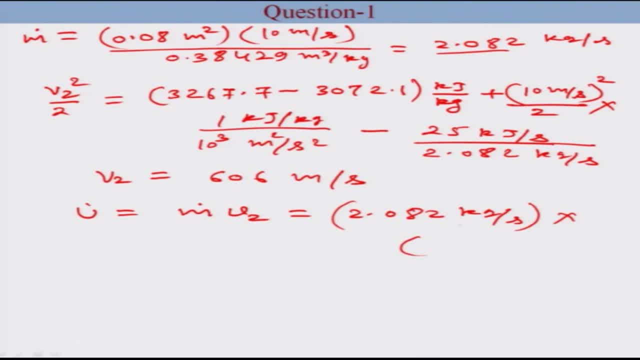 So now we have to calculate the volumetric flow rate at exit. So now we have to calculate the volumetric flow rate at exit. So after putting these values here, 2.082 kg per second by 2.082 kg per second, So from here we get volumetric flow rate V dot equal to 2.74 meter. 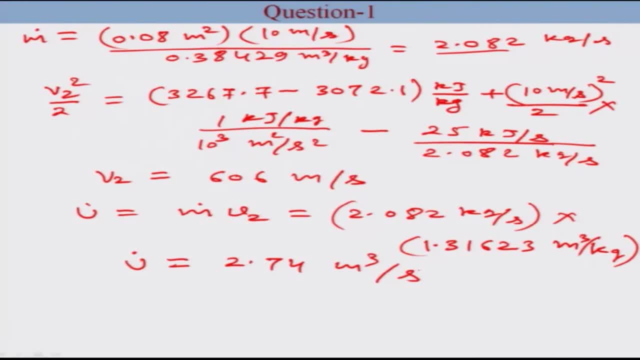 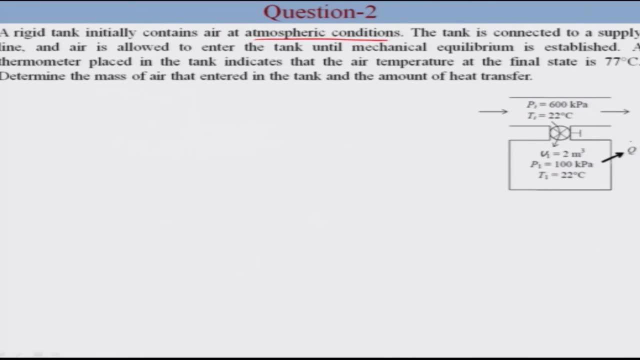 cube per second. So, moving to the next question, heat tank initially contains air at atmospheric conditions. The tank is connected to a supply line and air is allowed to enter the tank until mechanical equilibrium is established. A thermometer placed in the tank indicates that air temperature at the final state is. 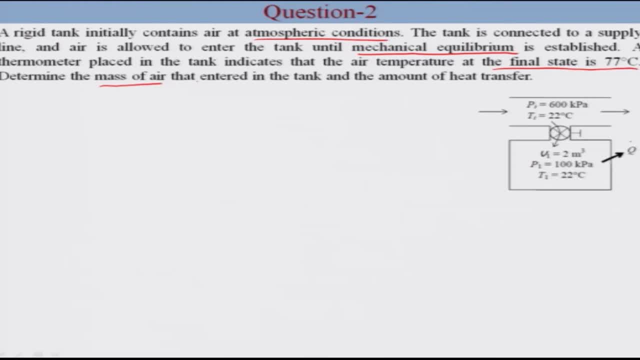 77 degree centigrade, Determine the mass of air that enter in the tank and the amount of heat transfer. So this is the sketch of the problem, and here we assume that this tank, as the system, which is a control volume, since mass is crossing the boundary. and here 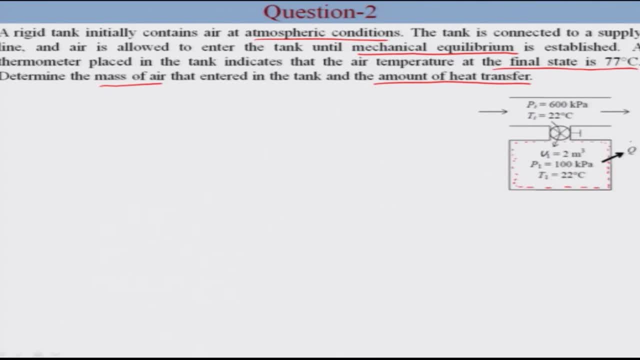 we need to find the amount of mass that has entered in the tank and total heat coming out of the system. So from the mass balance for this system we get mass coming in minus. total mass coming out of the system will be equal to delta m. 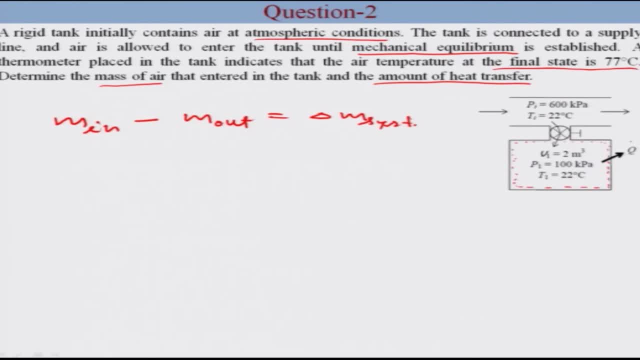 of the system. This is an unsteady state process but we can analyze as a uniform flow process since the state of the fluid at this inlet condition remains constant. So we will analyze it as a uniform flow process. Nothing is coming out of the system, so the mass out will be. 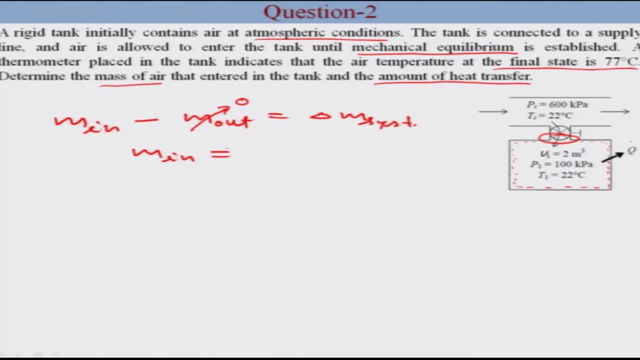 0.. From here mass in will be equal to change in mass of the system, which is m 2 minus m 1.. Now here we assume that air, as an ideal gas, initial and final mass of the air can. Initial and final mass of the air can be calculated as M1, equal to P1V upon RT1, ok. 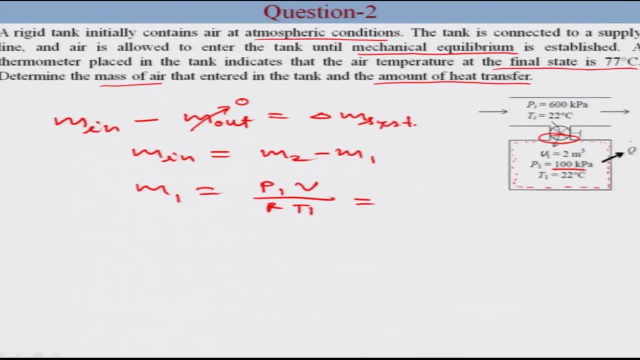 So P1 is given to us which is 100 kilo Pascal. volume of the tank is 2 meter cube and gas constant for air is 0.28 kilo Pascal meter cube per kg And temperature is 295 Kelvin correspond to 22 degree centigrade. ok, 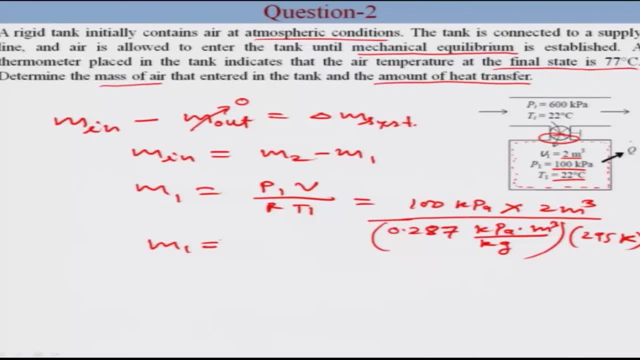 So M1, we will get here 2.362 kilo Pascal meter cube per kg. Ok, So M1, we will get here 2.362 kilo Pascal meter cube per kg. So M1, we will get here 2.362 kilo Pascal meter cube per kg. 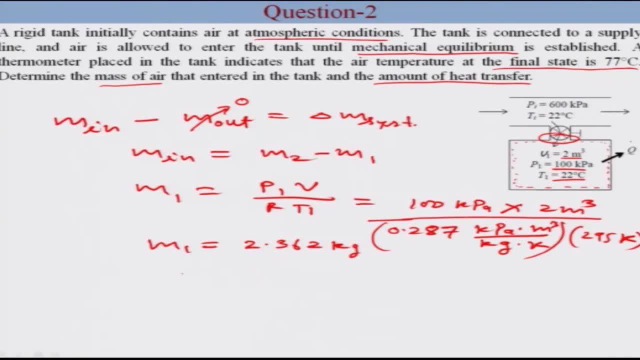 So, similarly, M2 will be P2V upon RT2, since the tank is rigid, so volume will be same. We need to find P2,, we do not do P2, but it is given that tank is in mechanical equilibrium with the supply line, ok, 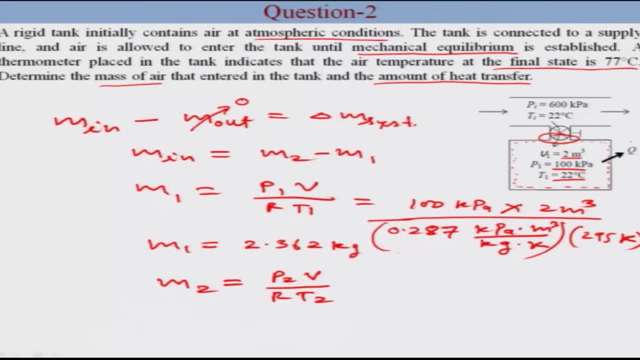 That means the pressure of the tank will be equal to pressure of the supply line, which is 0.. Ok, So P2V- the power increase of M2, is same, is 0.. S2 M2- the weight increase of the tank is 0. 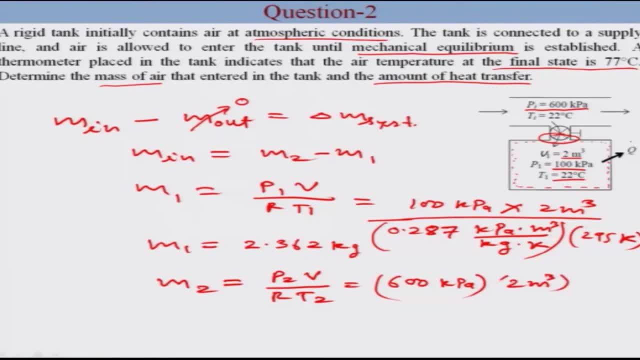 Soиж: 1.. Grease, snow volume, cool, proud pressure of a tank will be 0.. P2V is assigned 2 meter cube per 그리스र. 6антek Kilo Pascal meter cube per exec βC point. 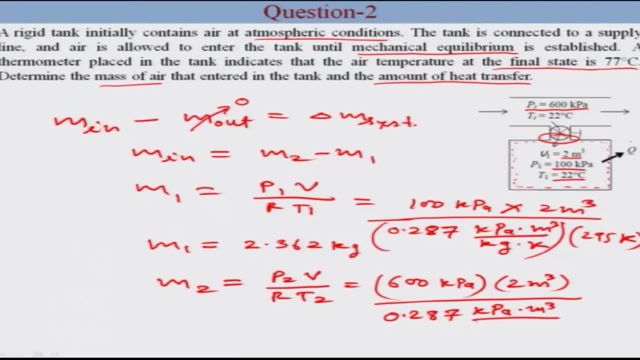 So putting this value here- 600 kilopascal volume is 2 meter cube upon- varies 0.287 kilo Pascal meter cube per Kelvin into 350 Kelvin. So this we will discuss later. it is 0.287 kilo Pascal meter cube per halogenuta Kelvin. 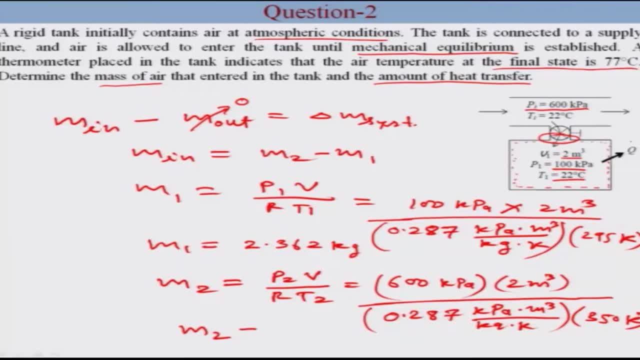 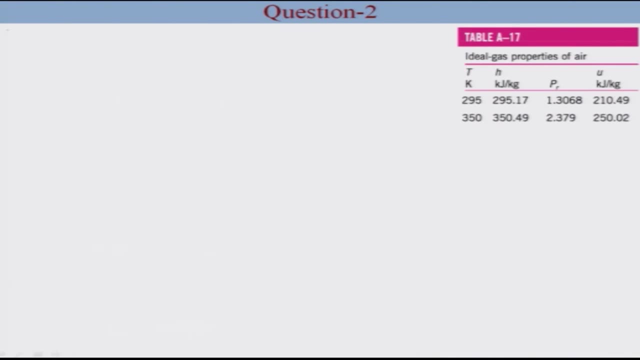 kilopascal meter cube per horse over 6 minute Kelvin. So from here m 2 would be equal to 11.946 kg. Now, further from the mass balance equation we get, amount of mass coming in the system will be equal to m 2 minus m 1, which is 9.584,. 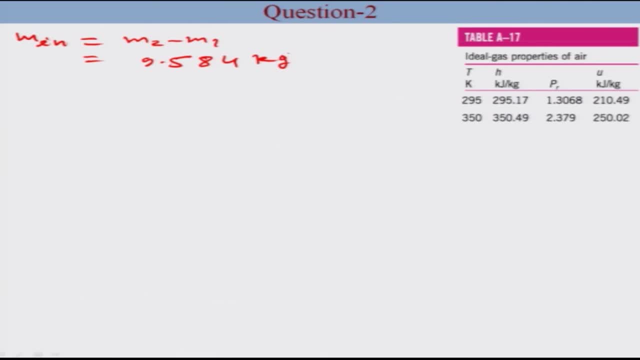 so this much of air will come into the system. Next we have to calculate amount of heat coming out of the system. So from energy balance, total energy in minus, total energy out, will be equal to delta E of the system. So total energy is heat coming in plus total. 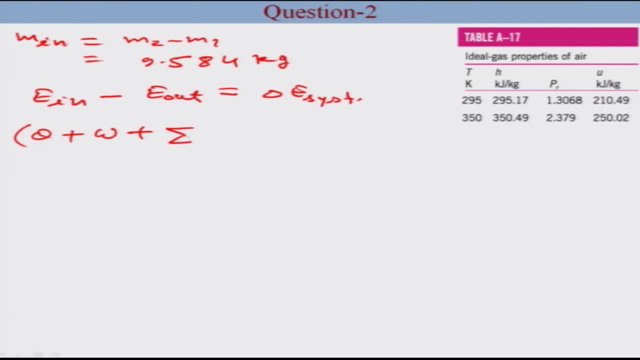 shaft work plus total heat coming out. So total flow energy of the fluid coming in the system minus total energy coming out of the system, which is Q plus shaft work plus total flow work of the fluid, which is equal to delta E of the system. 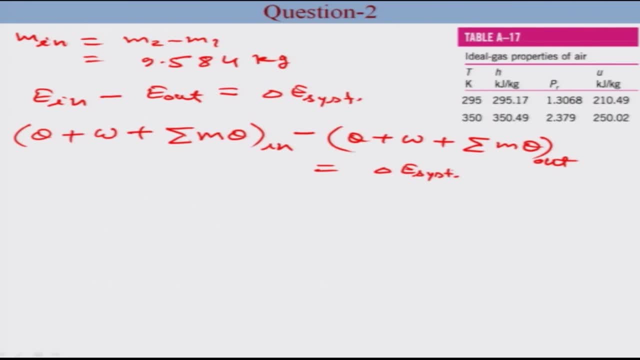 So we know that there is no heat coming in the system, no shaft work involved here and there is no work done by the system, So this will also be 0. and there is no flow work coming out of the system, So this will also be 0.. 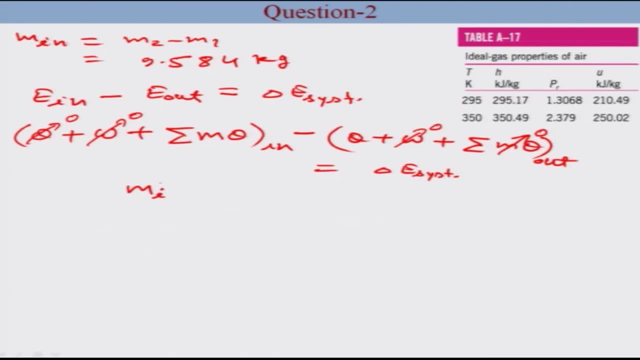 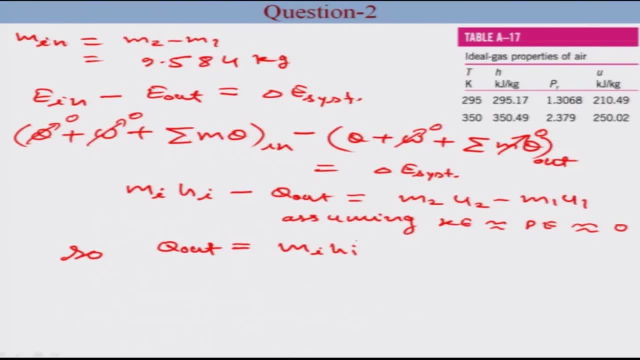 Mass coming in times: enthalpy coming in minus m 2, u 2 plus m 1 times u 1. so we have already calculated mass coming into the system. So after putting this value here, mass in is 9.584 kg per Xiao meter bred, lost, intelligent. 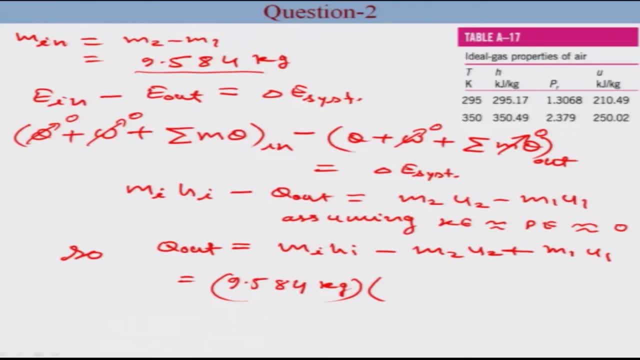 initial enthalpy is enthalpy at 295 kelvin because temperature is given initially. so initial enthalpy would be 295.17 kilo joule per kg minus m 2. that we have already calculated, which is 11.94, 6 kg times u 2. u 2 is the internal energy at 350 degree centigrade because the 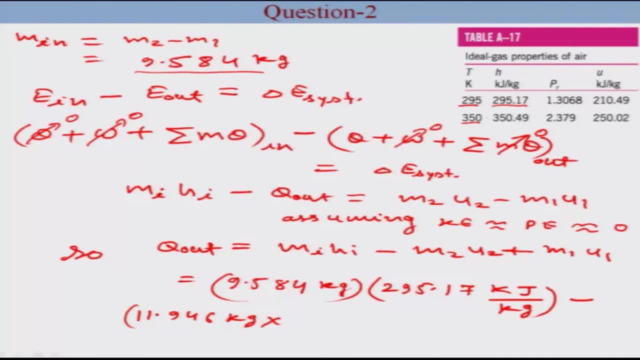 final temperature is 77 degree centigrade. so so u 2 will be corresponding to 350 kelvin, which is 250.02, 250.02 kilo joule per kg and m on plus u 1, m 1 is to point 362 kg times u 1. u 1 will 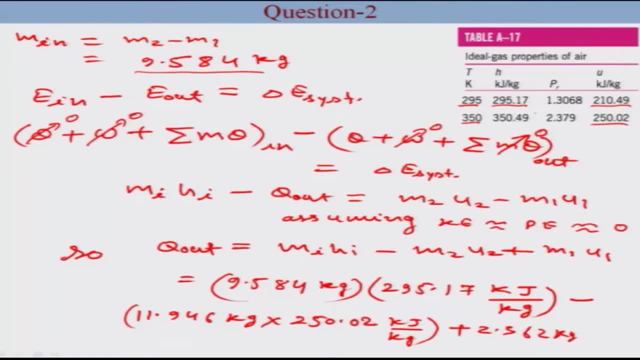 be the internal energy and 295 kelvin. so 210 point 49 kilo joule per kg and m one plus u 1 m 1 is 2.362 kg when we word it like this급 kilo joule per kg. ok, So after solving this we get heat coming out of the system equal. 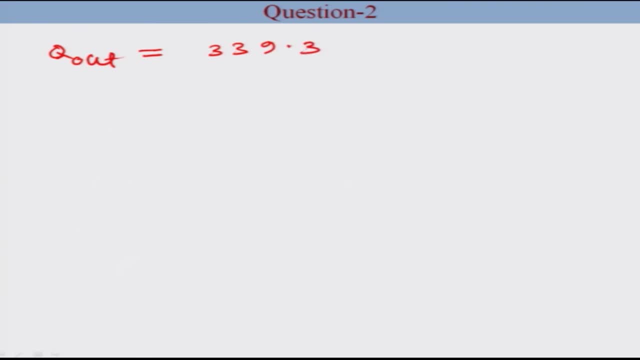 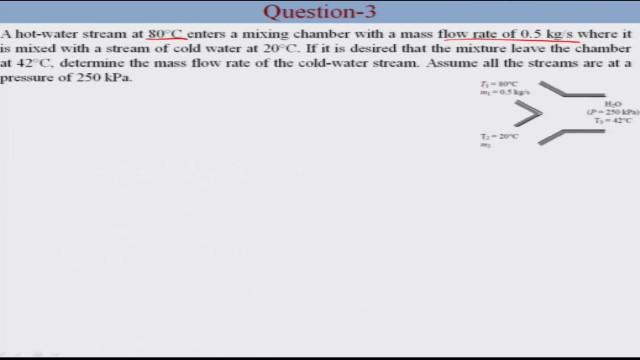 to 339.3 kilo joule. So, moving to the next question, a hot water stream at 80 degree centigrade enters a mixing chamber with a mass flow rate of 0.5 kg per second, where it is mixed with. 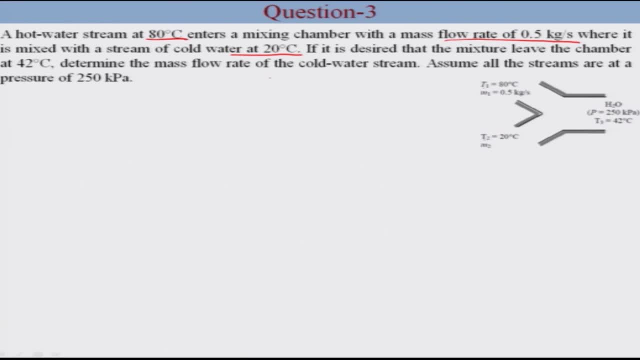 a stream of cold water at 20 degree centigrade, It is desired that the mixture leave the chamber at 42 degree centigrade. determine the mass flow rate of the cold water stream, assuming all the streams are at pressure of 250 kilo Pascal. So here we assume the mixing chamber. 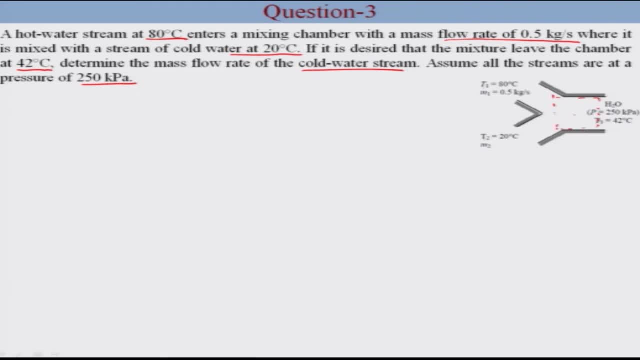 as the system and this is a control volume, since two streams are coming in to the system and one stream is coming going out of the system. ok, So from the mass balance of the system, total mass flow rate coming into the system minus total mass flow rate coming out. 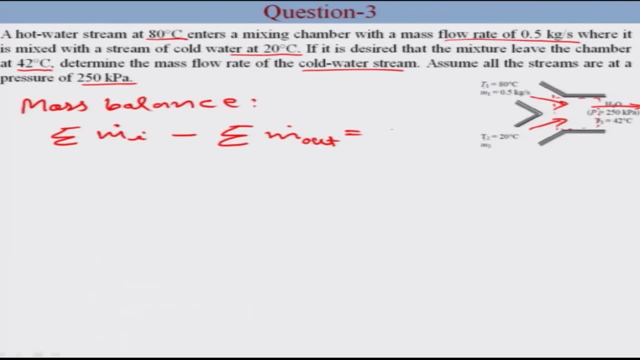 of the system will be equal to change of mass flow rate of this system. So this is what. So this is the steady state process, So nothing will change with time. So delta m dot will be 0. So from here we get m 1 dot plus m 2 dot will be equal to m 3 dot, because 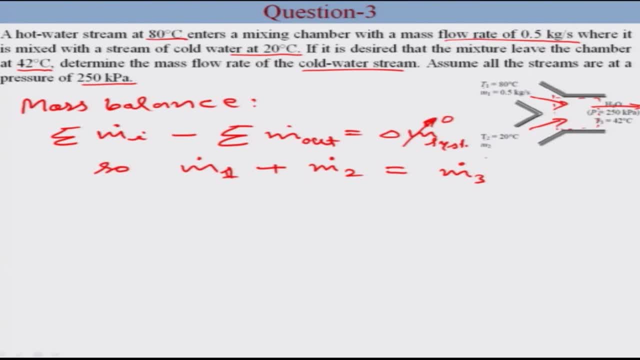 this is the only stream which is coming out of the system. From the energy balance we get rate of energy in, minus rate of energy out equal to change in energy of the system. So this will also be 0. So from here we get rate of energy. 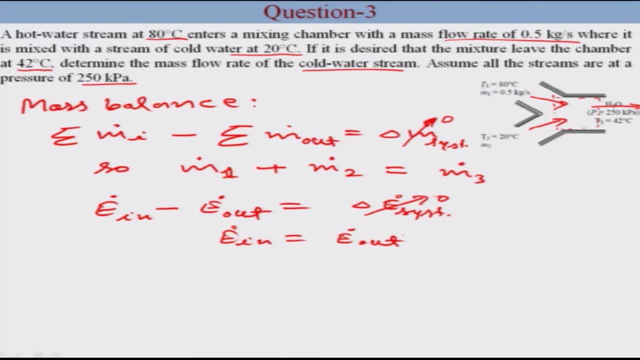 in will be equal to rate of energy out. Total energy in will be nothing but enthalpy of the first stream plus enthalpy of the second stream, which is going into the control volume, will be equal to enthalpy of the stream going out of the system. 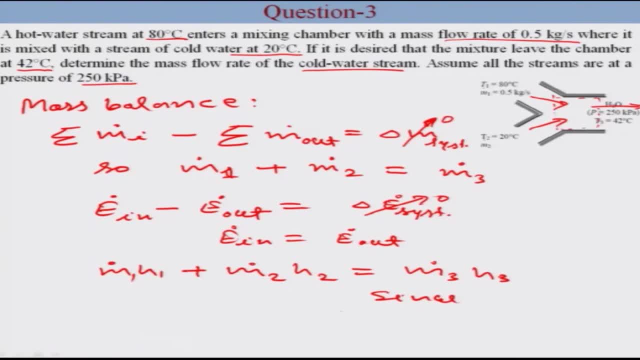 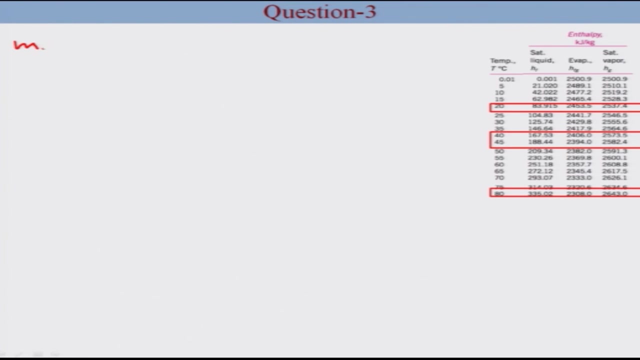 Since q dot, w dot and delta k e will be equal to m 1 dot plus m 2 dot will be equal to m 2 dot plus m 2 dot equal to delta p. we have assumed the f to be 0. So after combining this equation and this equation, we get m 2 dot equal to h 1 minus. 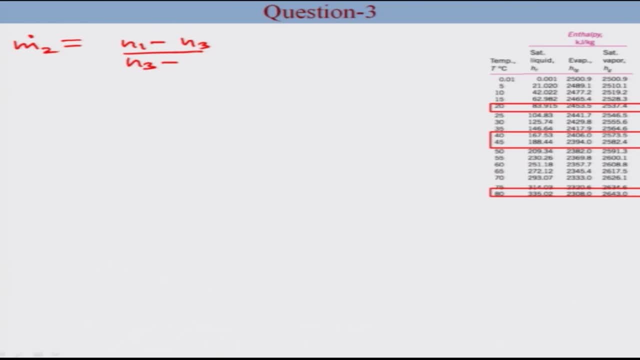 h 3 upon h 3 minus h 2 times initial mass flow rate. it Now to get the value of M 2 rod. we need to know all these variables Since it is given that all the streams are at 250 kilo Pascal, So at this 250 kilo Pascal of pressure. 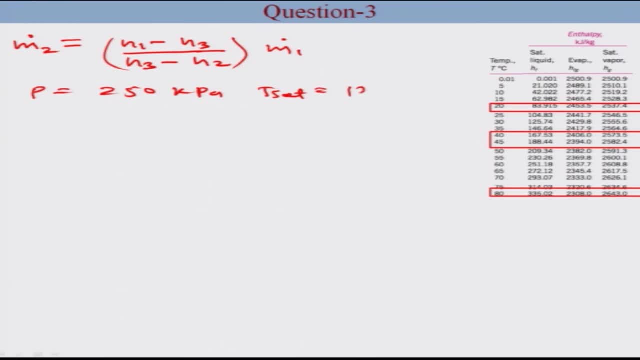 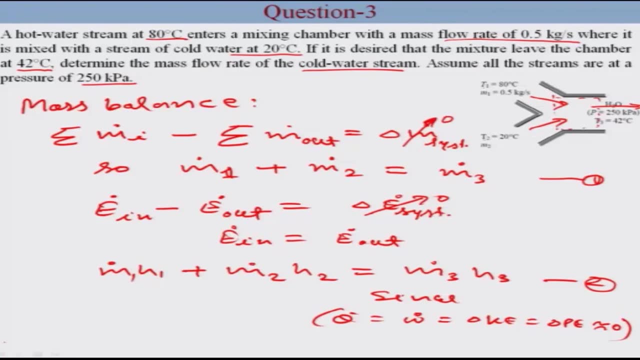 T saturation temperature should be 127.41 degree centigrade, but it is given that at this pressure temperature of all the streams are way below than 127.41 degree centigrade, which is 80 degree centigrade, 20 degree centigrade and 42 degree centigrade. That means all. 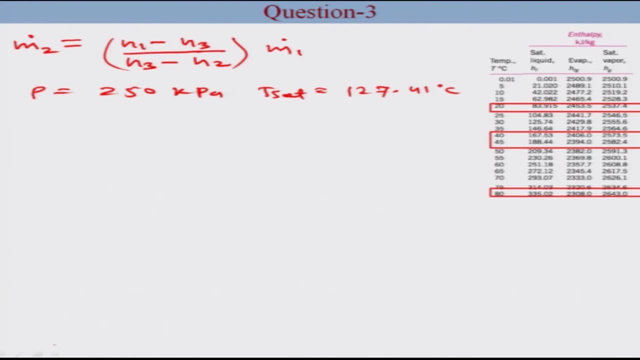 these streams are compressed streams which can be approximated as a saturated liquid at the given temperature. So in order to get enthalpy data we need to look into the saturated water table. So H 1 will be equal to enthalpy of fluid at 80 degree centigrade from the saturated 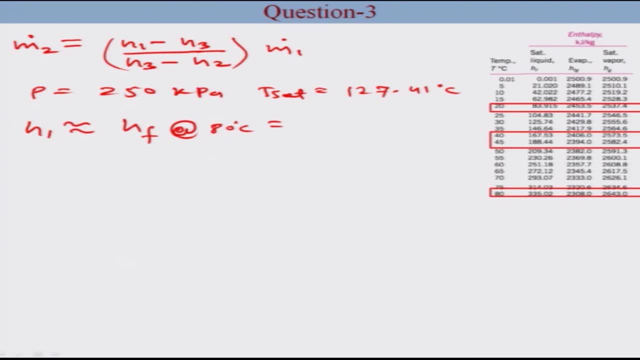 water table, which is listed here. So enthalpy would be 335.02 kilo joule per kg. H 2 will be 35.02 kilo joule per kg. Let us look at H 2.. So we have an enthalpy of the fluid at 20 degree centigrade, which